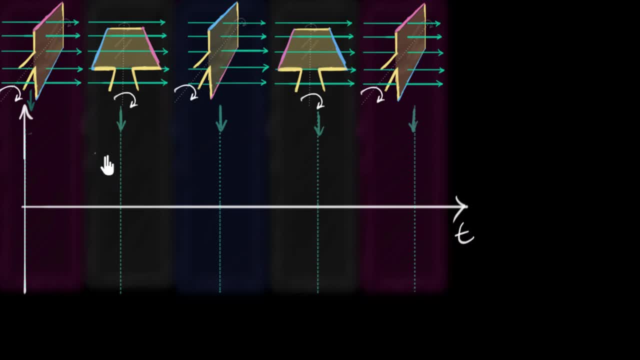 time Now. to do that, we need an equation connecting the flux and the time, And I encourage you to pause the video and figure out that equation yourself, because you probably already know how to calculate magnetic flux, Alright. So how do you calculate magnetic flux? We calculate magnetic flux as whenever. 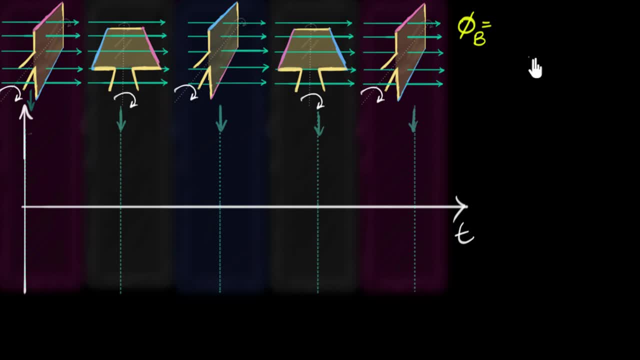 you have flat areas and uniform fields. we calculate as just N times the field strength, B times the area of the coil, A times cos of the angle between the magnetic field and the area And be very careful with that. So the angle theta is the angle between the 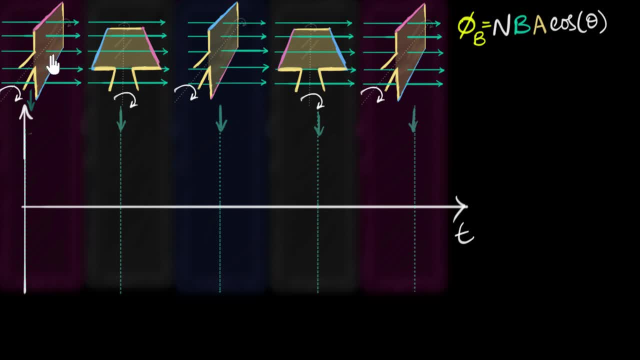 field vector and the area vector. Over here it looks like the angle is 90, but that's not theta. So you have to first draw an area vector, and if you draw that, the area vectors are always drawn perpendicular to the area. So we could draw an area vector like this And: 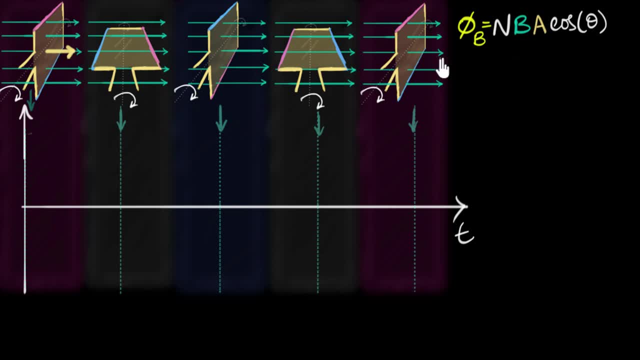 so notice, the angle over here is zero because they're both parallel. Okay, So this is zero angle. Alright, So we can draw the area vectors everywhere And then we can see what the angle between them is. And if I draw that over here, it 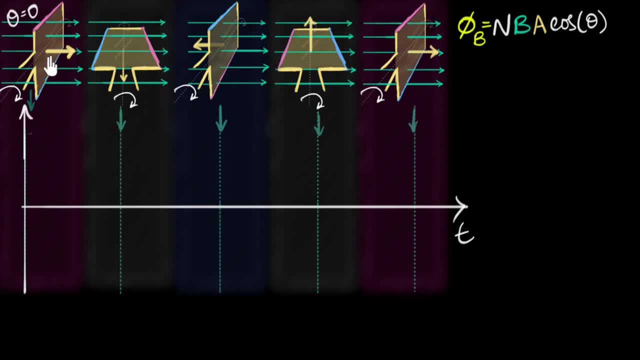 will be down. So let's draw that. See as it is spinning. the area vector is turning as well. So it's down, left comes up and comes to the left, right, And so the angle is clearly changing. Theta is changing with time and that's how the flux changes. So if 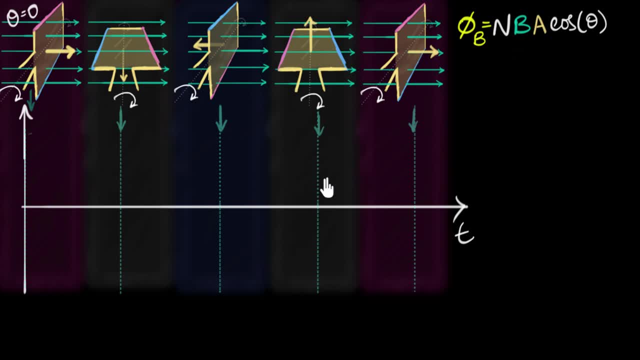 I can now figure out how theta is changing with time. I get my equation, I can plot. So how can I connect theta with respect to t? How can I make theta as a function of time? Well, this goes back to our rotation. Just like in linear motion we can say: distance covered equals speed into time In angular 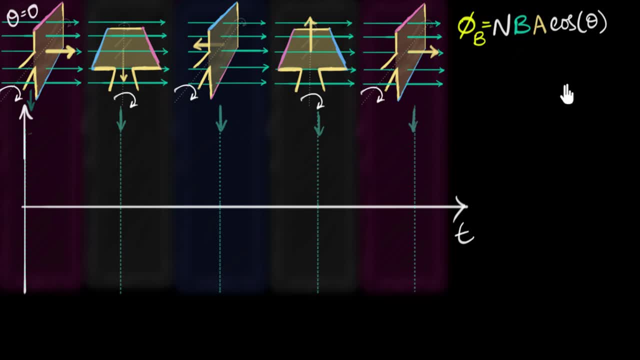 motion. we can say angles covered equals angular speed into time. So what we can do is let me rewrite this So we can write: phi b, oops, phi b equals nba times, cos of. I can say that angles covered equals angular speed into time, Just like distance equals speed times, times. 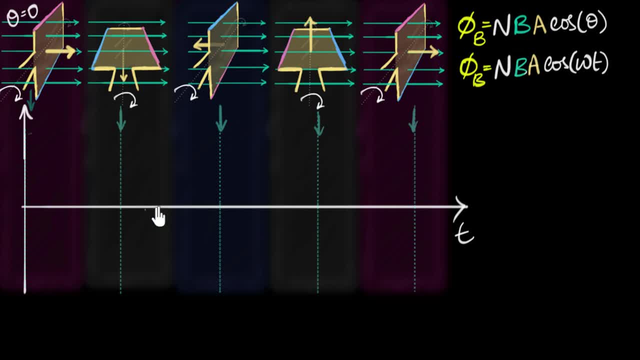 And now I can go ahead and plot this over here. So let's do that together. Let's first put some specific points. So let's say that this is the moment where t equal to zero, Just to keep things simple. So let's assume this is our time: t equal to zero. We start. 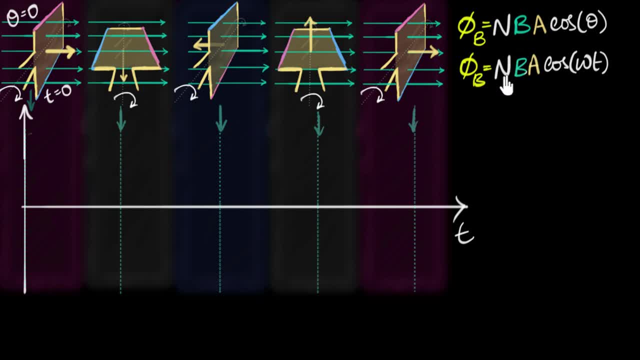 our clock at this point. So, right now, what is our flux? Well, right now, theta is zero. I can directly look at: theta is zero, Cos zero is one, And so the flux right now is going to be just nba. 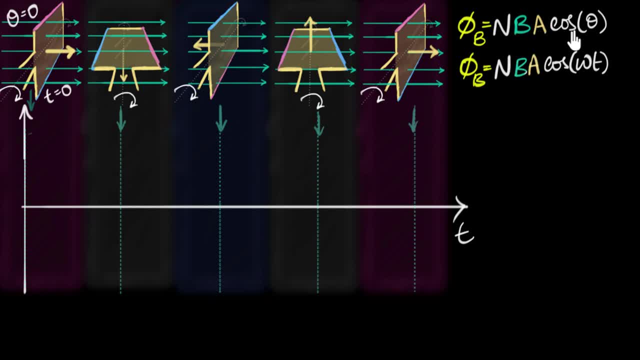 And guess what? this is the maximum flux you can ever get, Because the maximum value of cos is just one. And so if I call that maximum flux, this nba represents the maximum flux. If I call that as phi- you know I can just say phi naught- then right now at time, t equal. 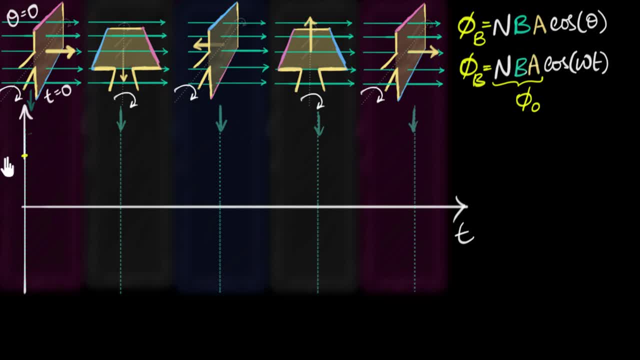 to zero, I get maximum value. So let's say this is our maximum value, This is our phi naught. Okay, what about at this position? What is the value of flux over here? Well notice, the angle between the area vector and the field vector is 90 degrees. So this is. 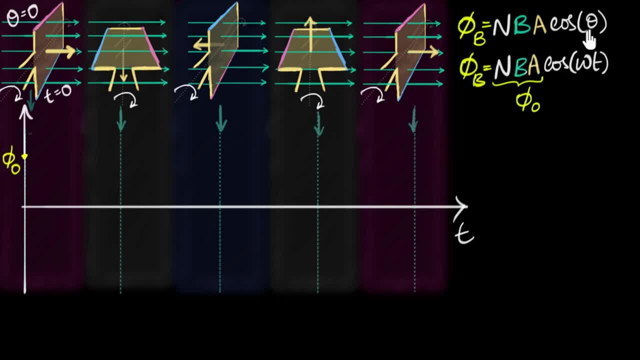 90 degrees, Cos 90 would be zero, right? So I can just look at this. I know the angle immediately is 90 degrees. the angle turned angle between the area vector and the field vector is 90 degrees. So cos 90 is zero. So I get zero flux at this point. 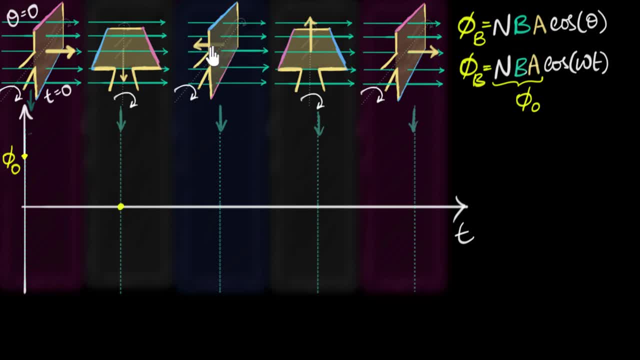 What about over here? the angle between the area vector and the field vector is 180 degrees, And therefore I get negative one. cos 180 is negative one, And so I get flux equals negative maximum, And so it will be somewhere over here. You may be wondering what does it mean to have? 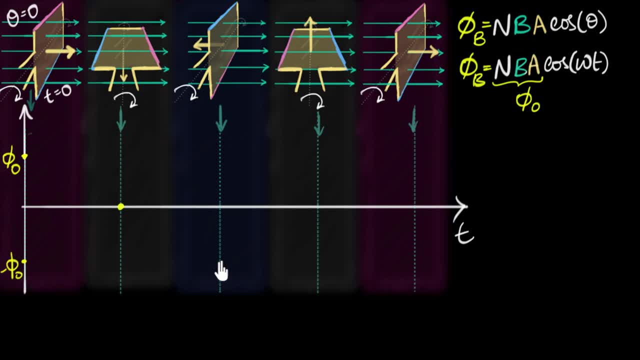 a negative flux. What does that mean? Well, the way to think about it is: you can imagine that this window has an orientation. So in this case, you can kind of imagine if the window, if the air, was flowing in one direction. when the window has turned by 180 degrees, 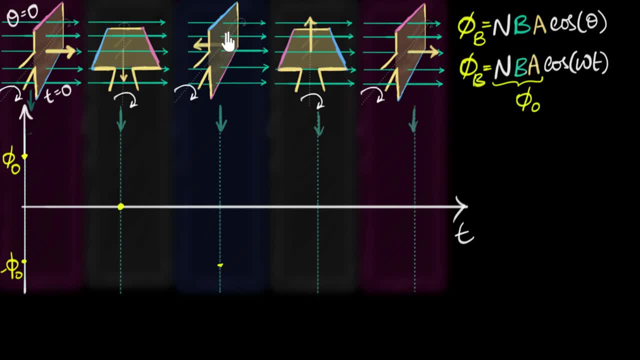 now it's facing the other way, So from the windows perspective, the air is flowing in the opposite direction. Does that make sense? And so that's why we say there's a negative flux. So this is positive flux, this is negative flux. 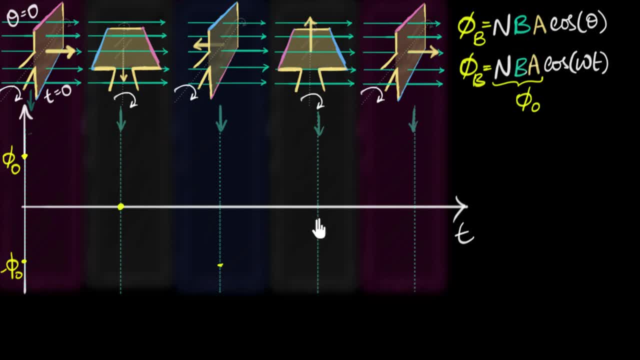 Over here the flux becomes zero again And finally, over here the flux back goes back to maximum. So how would that flux, How would this whole thing look like? Would it be just like straight lines? No, it's a cos function And you might know cos and sine functions. 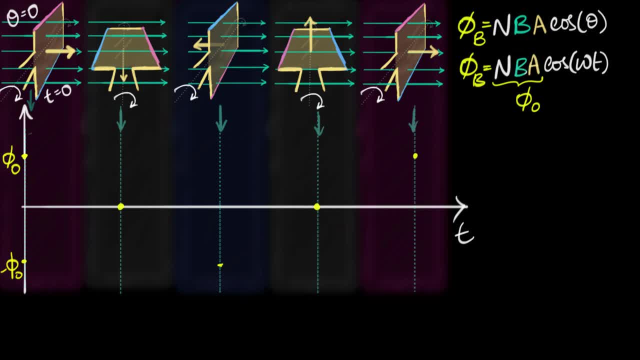 have that typical graph, So let's go ahead and try and plot that graph. So the typical graph looks like a wave. So it's going to look like somewhat like this: Okay Okay, Okay, Not quite there, but yeah, Not bad. Looks pretty good, right. Next we will do the same. 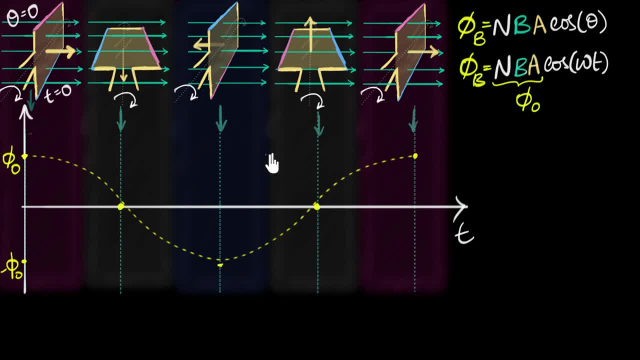 thing for the EMF. We'll figure out the equation for the induced EMF and then plot the graph. But before we do that, I want you to make a prediction of how that graph is going to look like. Remember, the EMF induced is high when the flux change is very high, And so 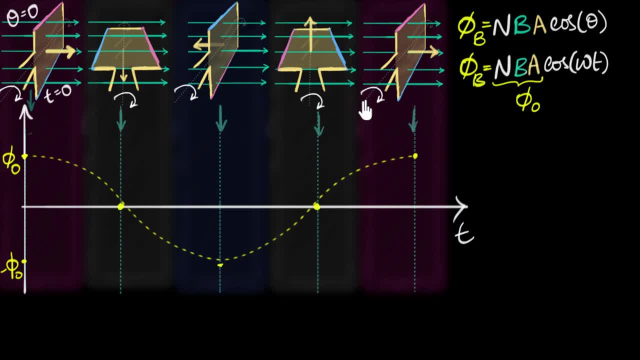 at each point. can you kind of predict whether you get a high EMF or low induced EMF or zero EMF, And kind of predict what the graph is going to look like? Okay, Hopefully you made your prediction. Now let's check whether you know whether it matches. So let's build. 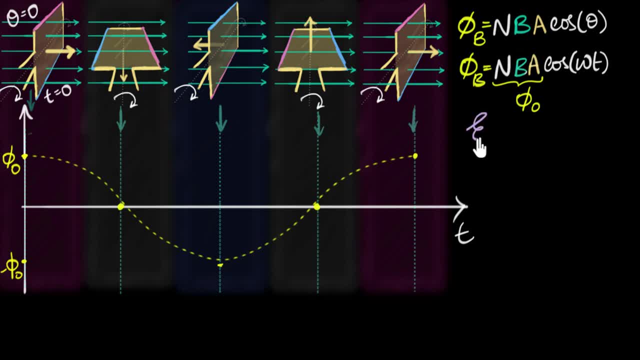 the equation. How do we build the equation? We can use Faraday's law. Faraday's law states: the induced EMF is always equals negative d phi, d phi over dt, And so all we have to do is differentiate this equation with respect to time And again. I encourage you to try. 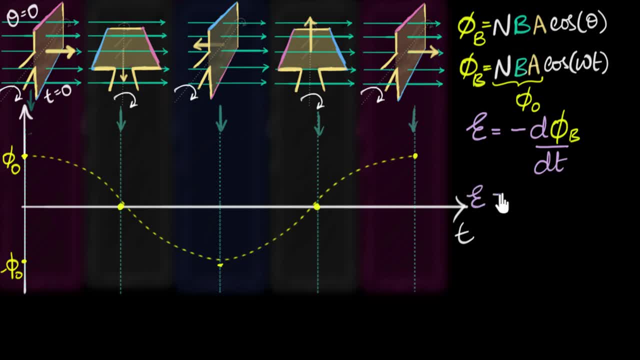 and do this yourself. So let's do this. So the induced EMF will be negative. What's the differentiation of this term? Well, n b, a are all constants. We can pull them out, So you get n b a over. 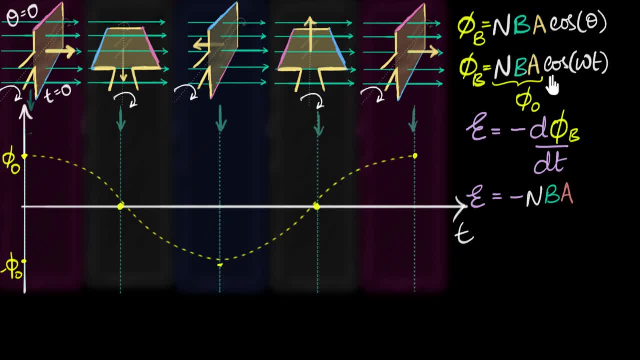 here, And then you get differentiation of cos, omega t. Differentiation of cos is negative sine, So minus sine, omega t. And then you have to use a chain rule. Then multiply by differentiation of omega t, which gives you an omega, So an omega pops out. And so if 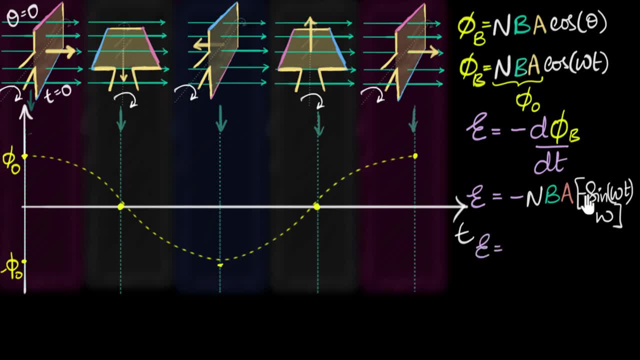 you put it all together, we now get EMF equals, negative, negative cancels. So I get n b a n b times a times omega times sine of omega t, which is basically the angle. And there we go. This is the expression for the EMF And, just like before, this now represents: 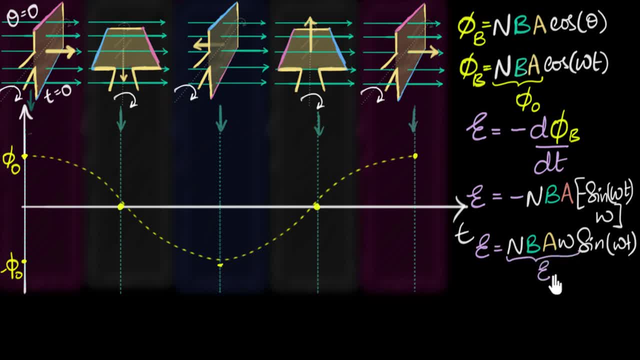 the maximum induced EMF, which you can call E, nought, E nought. So now we know what the induced EMF depends on. It depends upon the number of turns, the strength of the field, the area of the coil and how quickly you're spinning it. The quicker 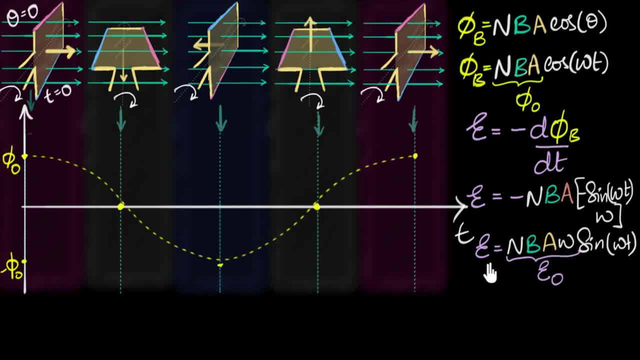 you spin, the more quickly the flux changes and higher is the induced EMF. Okay, now let's go ahead and plot this over here. So, and when omega t equal to zero, when t equal to zero, when theta is zero, sine zero is zero. so you get induced EMF at this position is. 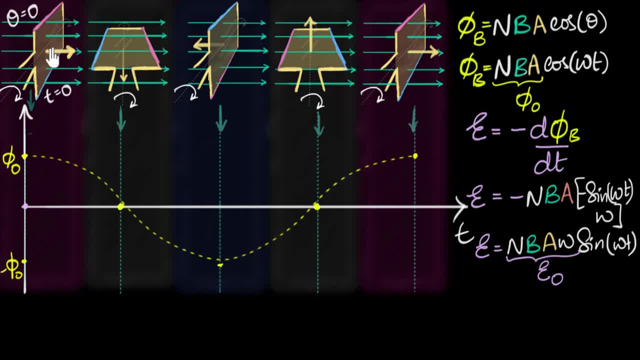 zero Interesting. Did you predict that At this point you get zero EMF in this position? Okay, Then, after it has turned through 90 degrees, sine 90 is one. So now you get maximum EMF at this position. So let's say this is our maximum EMF, And so the maximum EMF will be somewhere. 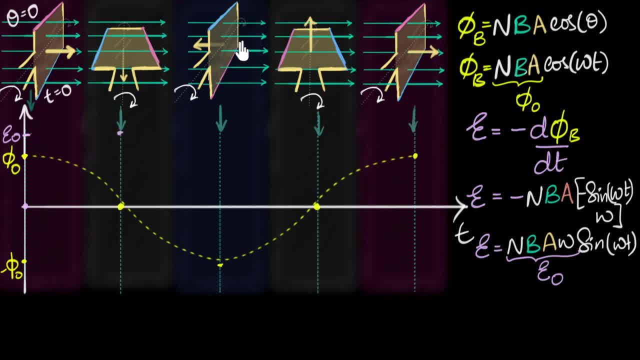 over here, Then at this position it has turned by an angle of 180 degrees, And so now you get sine 180 is again zero. So you get zero here, And then at this point you would have turned by 270 degrees. Sine 270 is minus one, And 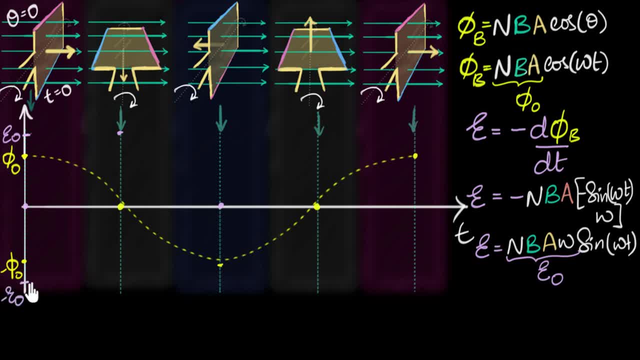 so you get now negative maximum, So you get somewhere over here, And finally by the time you come here you would have turned by a whole 360 degrees. Sine 360 or two pi is zero, And so EMF becomes zero again. So you have to plot that. Let's do this. Another sine wave is going to look like this: 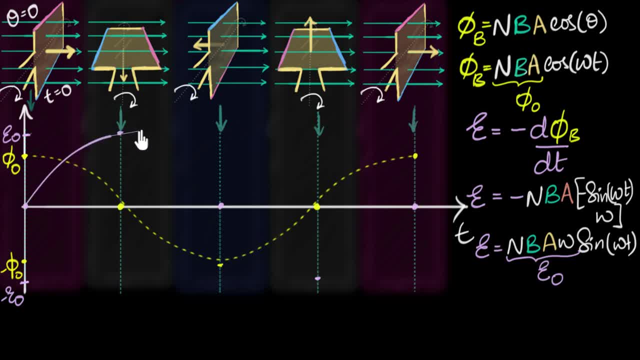 Another sine wave is going to look like this. Another sine wave is going to look somewhat like this, And so our EMF also is a sine graph. It can fluctuates between positive E naught and negative E naught, And that's why we say it's an alternating voltage. 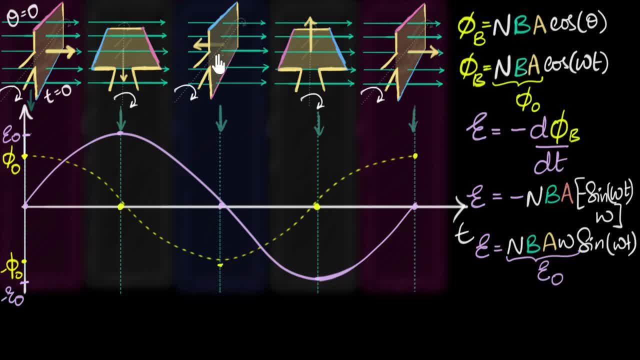 So how long does it take to go from here to here? Well, it depends upon how long it takes to finish a rotation. So if you spin this a hundred times per second, then our EMF will alternate between plus E naught and minus E naught a hundred times per second. And this 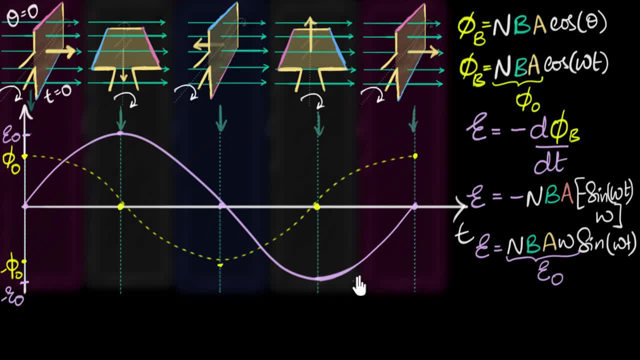 is what we call the frequency. In India, the frequency is close to 50 hertz, which means the coils will be spun at 50 times per second, And so our EMF will also alternate at 50 times per second. Finally, one peculiar thing that you're seeing is that 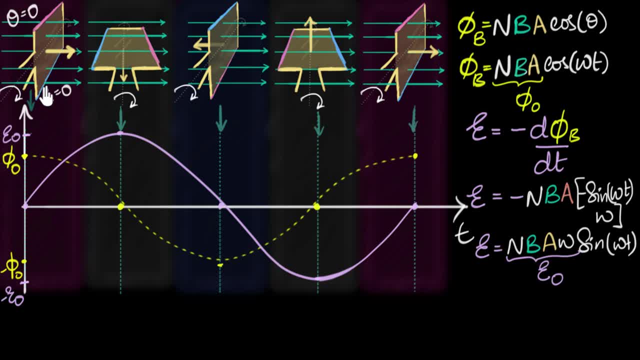 at this point, where the flux is maximum, I'm getting zero EMF, And when the flux is zero, I'm getting maximum EMF. What's going on? I would have predicted exactly the other way around. What do you think is going on? Well, Faraday reminds us. I don't care about flux. 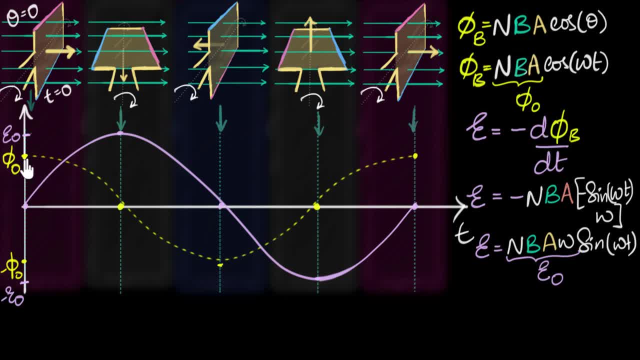 I care about the flux change. Okay, So at this point, if you consider this like a mountain, then the height represents the flux. Faraday is saying: I don't care about the height, Tell me how quickly the height is changing. So imagine you're standing somewhere. 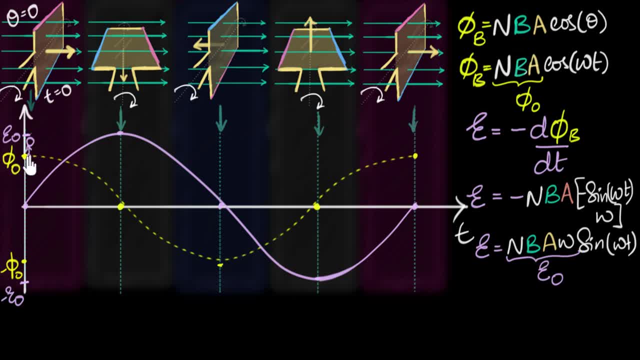 over here. How steep is this? It's not very steep, It's very flat, isn't it? So the slope over here is zero. You put one step forward, you don't immediately fall down. It looks very flat to you And therefore the flux is not changing very quickly at this point. 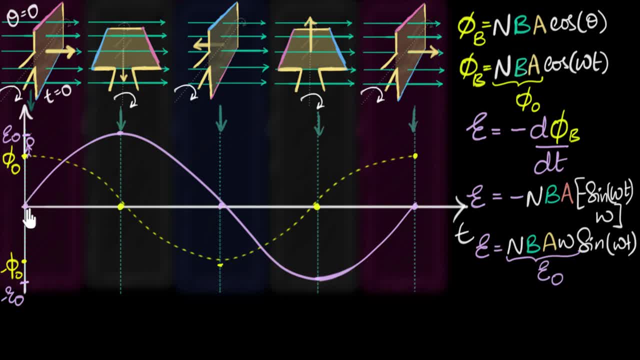 Slope is zero And that's why the EMF at this point is zero. Okay, What about this point? At this point, although the flux is zero, if you stand over here, notice it's very steep, very, very steep. You put one step forward and you go immediately down. So clearly there's 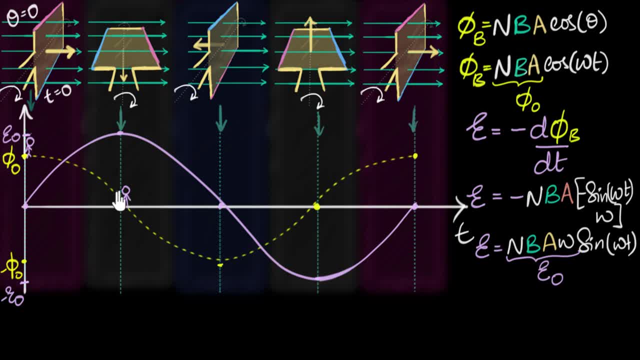 a very high negative slope over here And that's why we're getting a very high positive EMF induced. Why? Because of the minus sign Lenz's law. If the flux is changing, if the duct is decreasing, EMF is trying to increase the flux and you're getting a positive EMF. 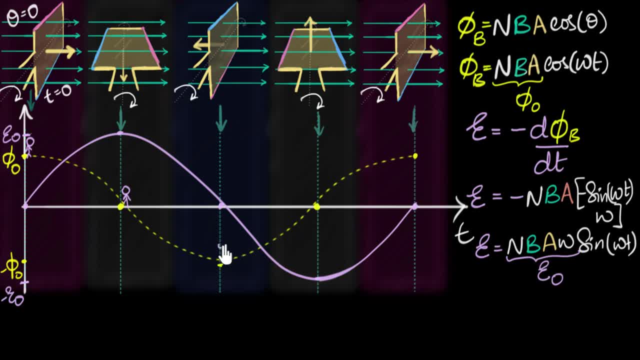 Ooh, it's all trying to move. Makes sense. Same thing happens over here. At this point you have a very high negative flux, but look at the change. It's nothing. You can stand here easily. There's no slope. 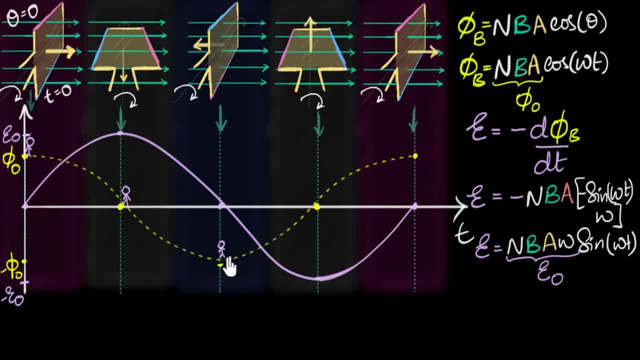 You put one step forward, hardly there is any change in the height And therefore EMF induced is zero. And the same thing over here. If you stand over here, ooh, look at the slope- Very high, You know it's a very steep thing. You put one step forward, you go high tremendously.